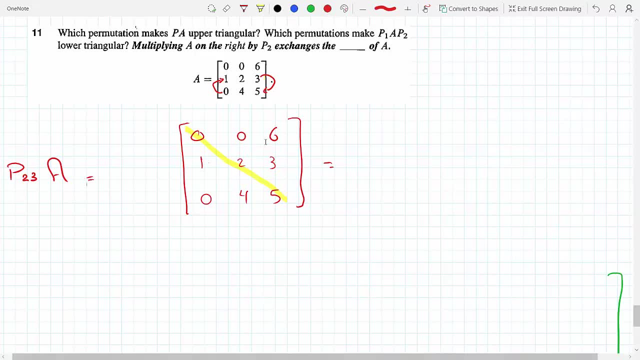 And so that means let me take this a little bit To the left, To the right I mean, because I have to pre-multiply it. So P23 is the identity matrix, with rows two and three switched. So first row is the same one, zero, zero. 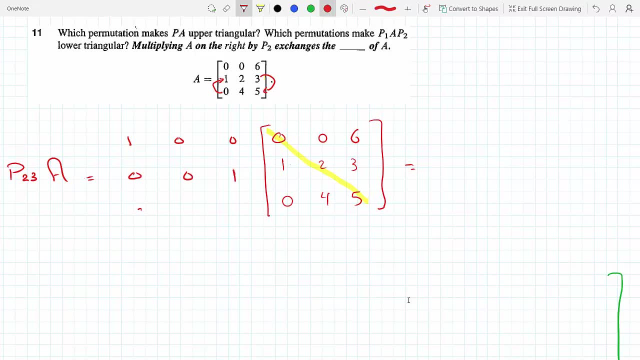 And then the second row would be zero, zero, one, And the third row would be zero one, zero. And if I do that, the effect that this have on the result is that the two rows, two and three, of A will be switched. 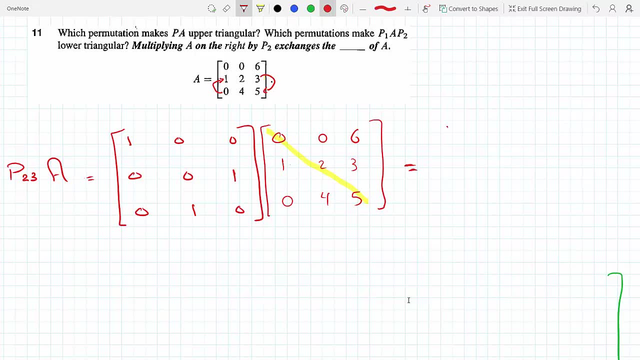 So the end result will be zero, zero, six. This one doesn't change. And then here I have zero, four, five and one, two, three. Okay, now I would need this first row here to go to the last. 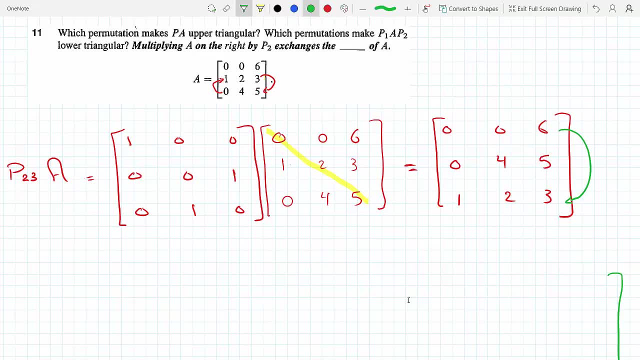 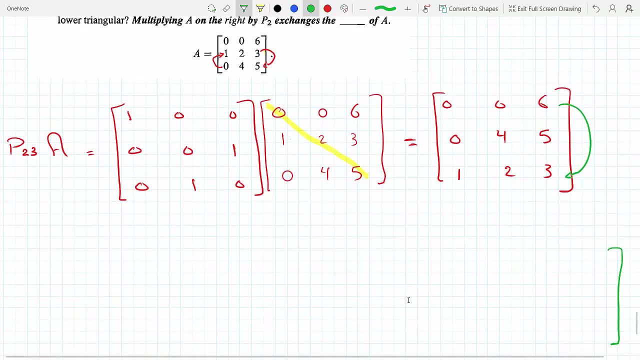 Or sorry, yeah, an upper triangular. So I need to switch row one and row three. So I would have to take the result, which is P23 times A, And I would have to multiply it by the permutation one three, One, three. 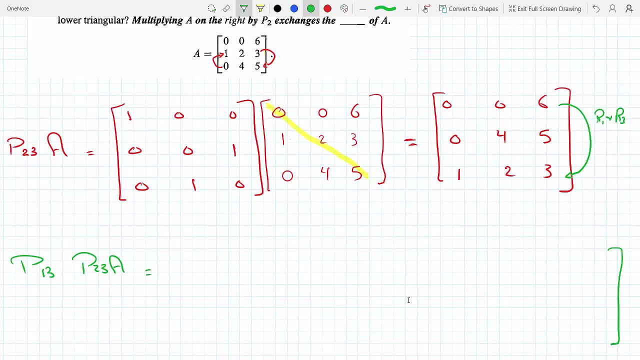 Row one switched with row three, So that would be zero, zero, one. The third row, So this P13 is the identity matrix, with rows one and three switched, So zero, one, zero And one zero zero. And then I would pre-multiply this by the result that I got. 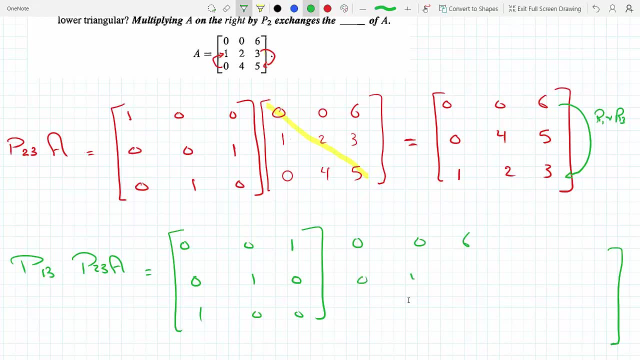 Zero, zero, six, Zero, four, five, One, two, three, And if I do this I will get exactly a lower triangular. This row three will go to the bottom And you can test it out if you don't believe me. 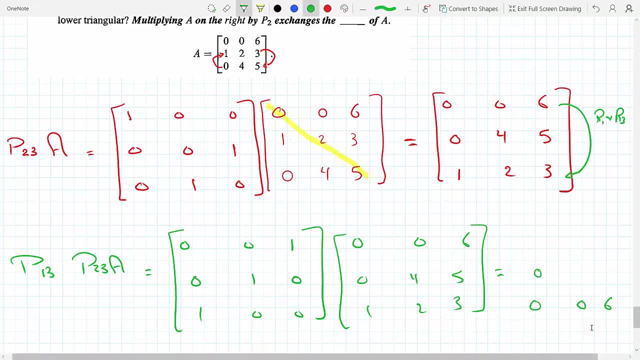 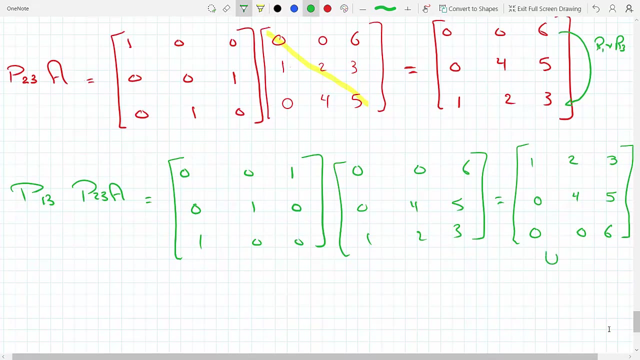 Zero, zero, six here, And then I would get zero, four, five unchanged, And then the one, two, three. This is an upper triangular, Upper triangular matrix. Now, what is it that I did? What is that matrix then? 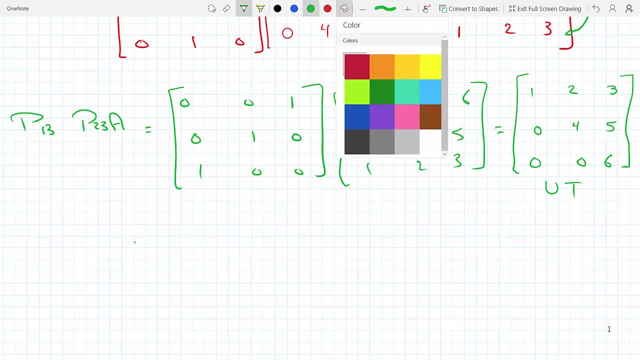 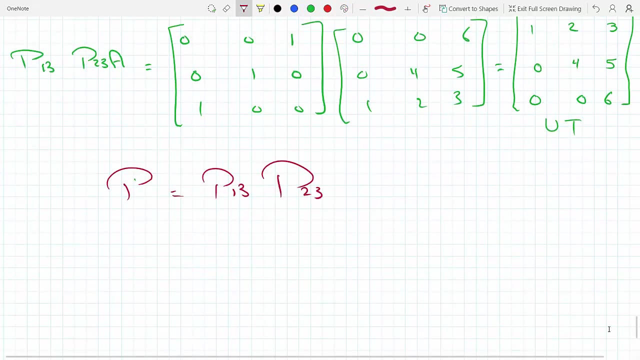 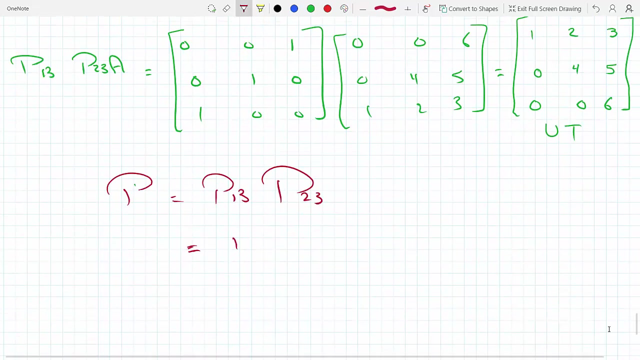 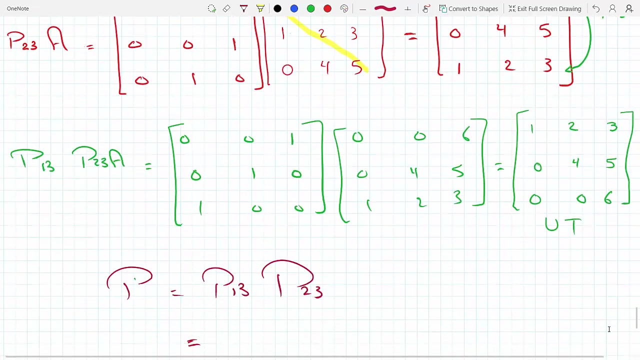 To answer the question. So the permutation matrix is P13 times P23. that operated on A to give me an upper triangular matrix. So one, three was one zero. so this is switched: One, three, two, three. Yeah, 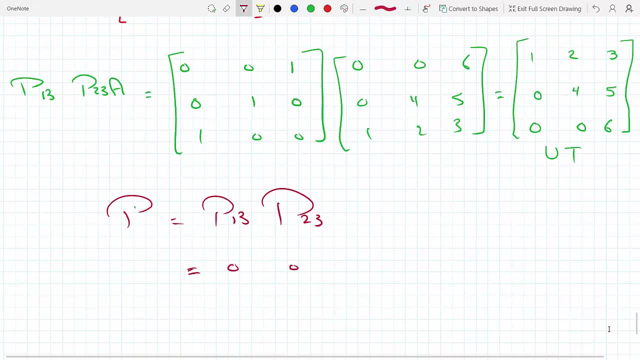 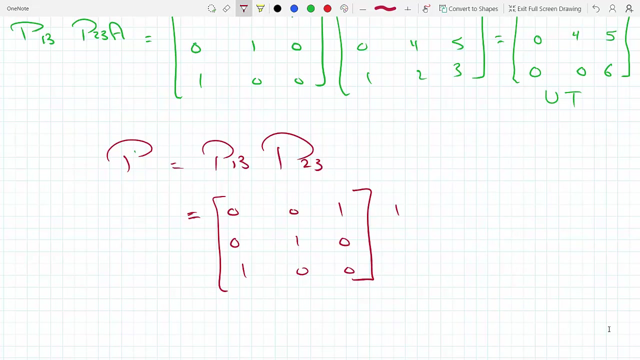 This is zero, zero, one Zero, one zero and one zero zero. So this is where the first and third row are switched, And here I have one zero, zero, zero, zero, one, two and three and then zero, one zero. 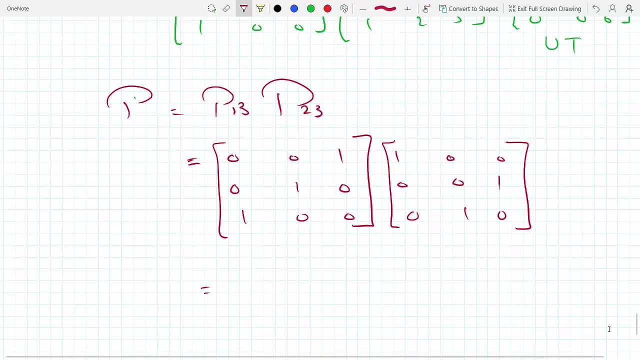 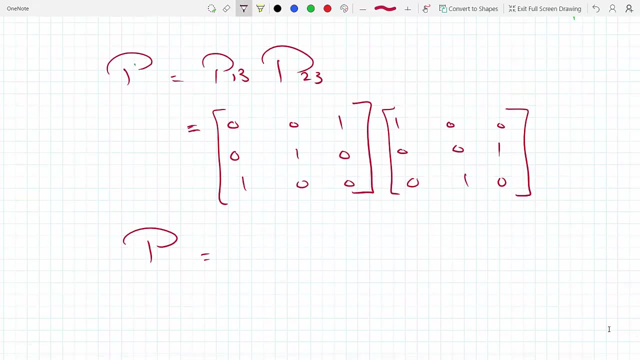 And then let's see what we get here. So of course, when you multiply two permutation matrices, you do get a permutation matrix. So I get zero, zero, zero, zero. So this is zero, This here is a one. So I know that the third cell has to be a zero because it has to be an identity matrix. 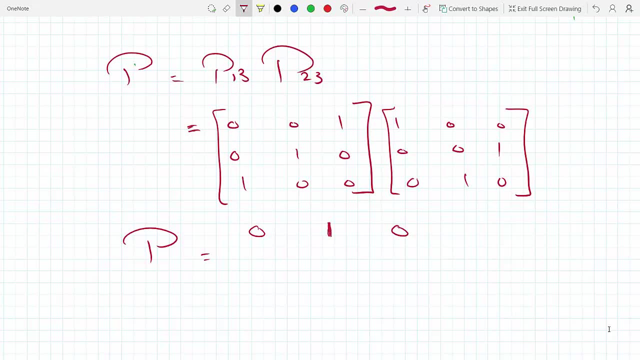 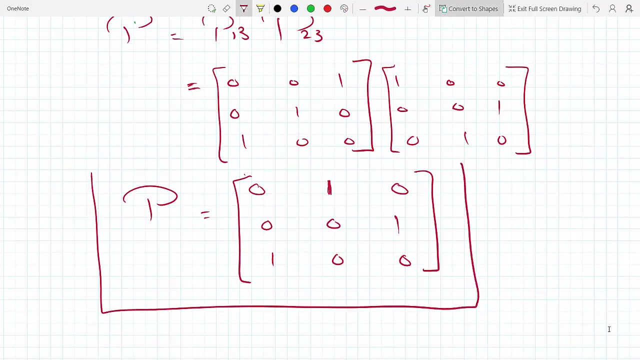 Yeah, Zero, zero. So this is a one, and which makes the third row one zero, zero. Yeah, I was doing the thing. What's that? So this is our permutation matrix to make it upper triangular. That answers the first part of the question. 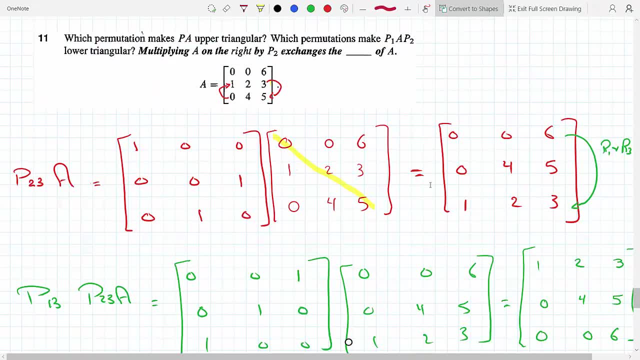 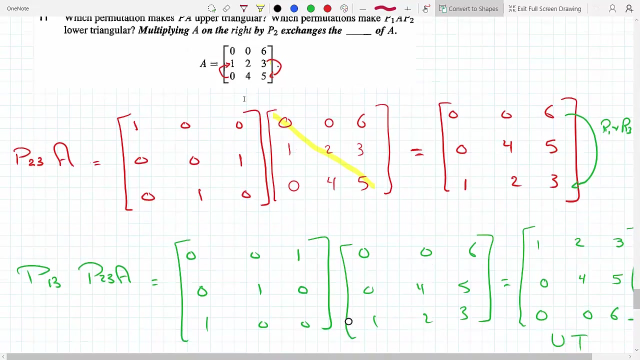 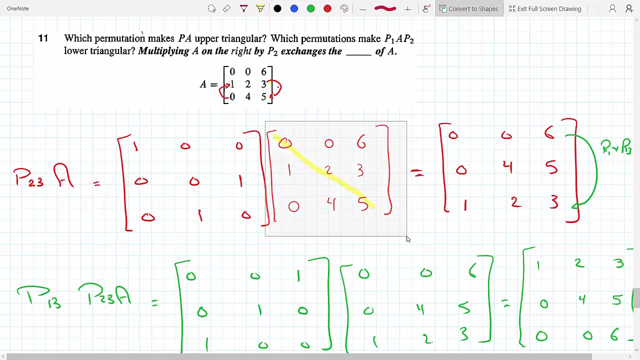 Okay, Part B wants this, or the second part of the question wants this: a lower triangular, Um And Uh. Two, make it a lower triangular. first we need to switch or exchange rows two and three. let me, and I want to copy and paste a here, the original, this guy, so copy so. 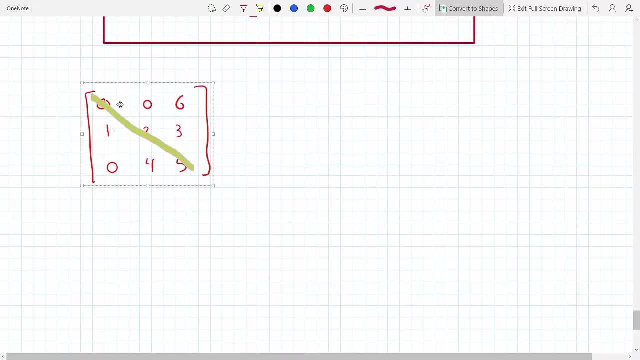 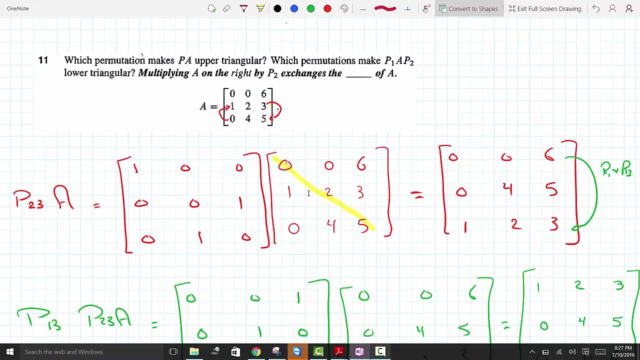 work it out here now. this is the second part, and let's move it to the middle a little bit, okay. okay, so I want this to be: what do you mean me? matrix P 1 times a times B 2? the way they have it, It means P1 first times A. matrix A times matrix P2.. 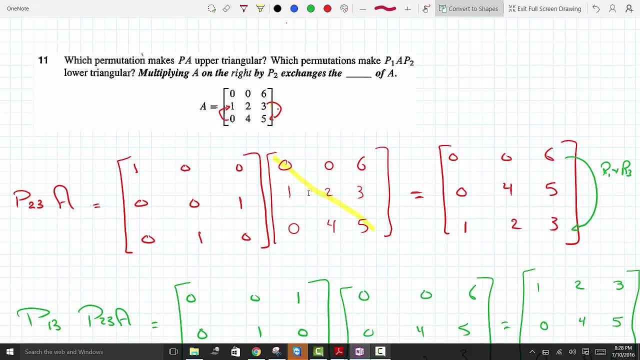 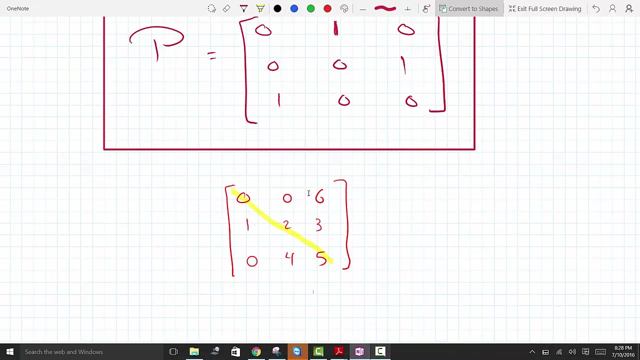 No, it doesn't, No, it shouldn't. Okay. So here we have to exchange row 2 and 3.. So here we have to exchange row 2, and So here we have to exchange row 2, and So here we have to exchange row 2 and 3.. So I can take that 0 up there, because the lower triangular, meaning everything above the yellow diagonal, has to be zeros. 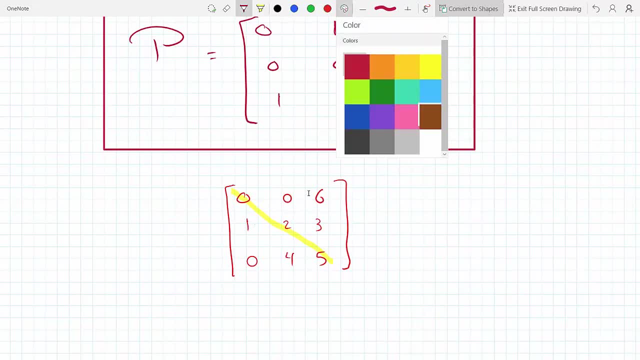 Okay, So now, then let me exchange this with this, and this has to go here. So what I have to do to this matrix A? then I would have to multiply it by P13.. So what I have to do to this matrix A? then I would have to multiply it by P13 times A. permutation 1,, 3,, oh sorry, P23 to switch the second and third rows. 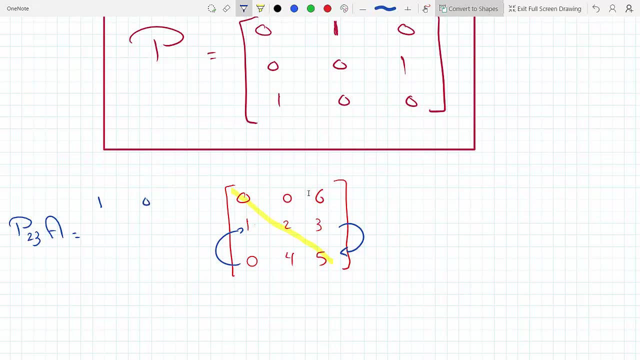 So I would do 1, 0, 0 and then 0, 0, 1 and 0, 1, 0. And if I do that- as promised you guys could try it out- You get 0, 0, 6 and these two rows get switched. 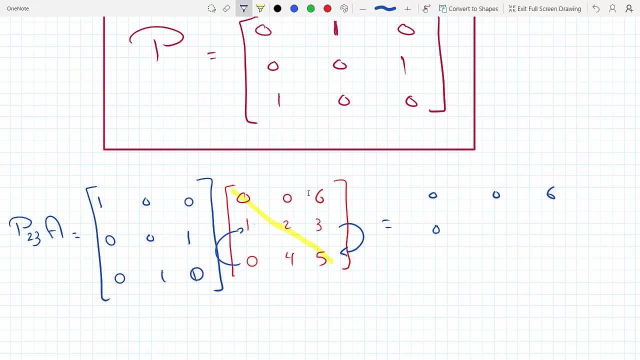 So I would have here 0,, 4, 5 and 1,, 2, 3.. Okay, Notice that the diagonal here is not in the right place. I'd want the diagonal to be right here. However, if you look, the diagonal is kind of swapped. 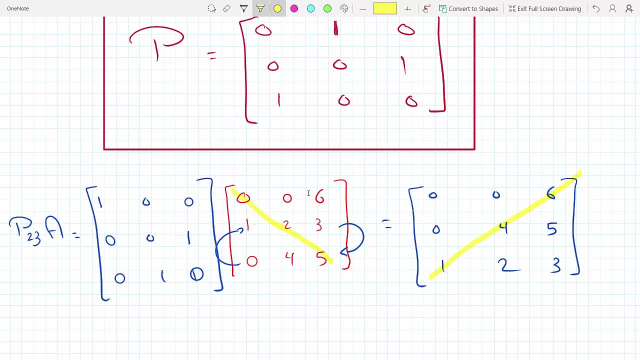 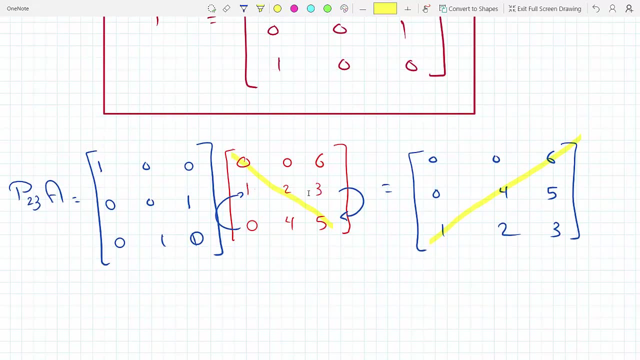 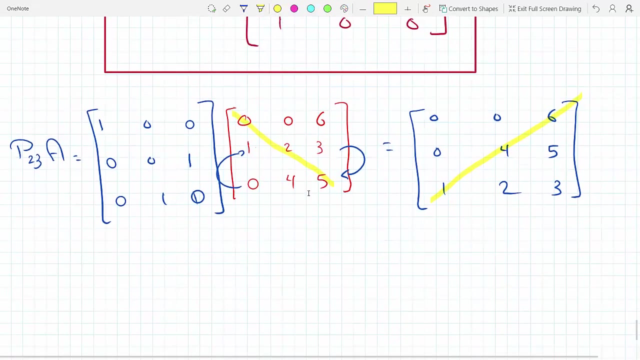 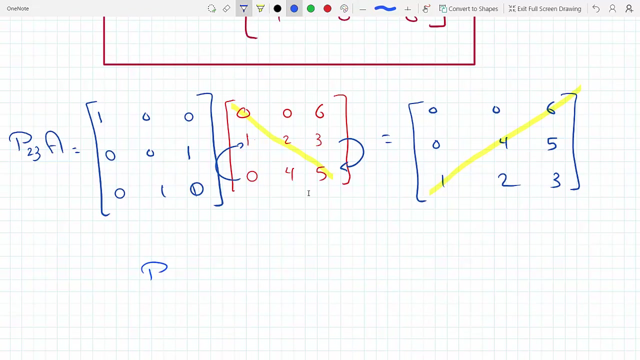 It's switched, It's on the other side. So what I need to do is I need to exchange the columns of A, And the way I would do this is I would take the end result, which is P23 times A, And I would multiply on the right-hand side, because multiplying A on the right would exchange the columns of A. 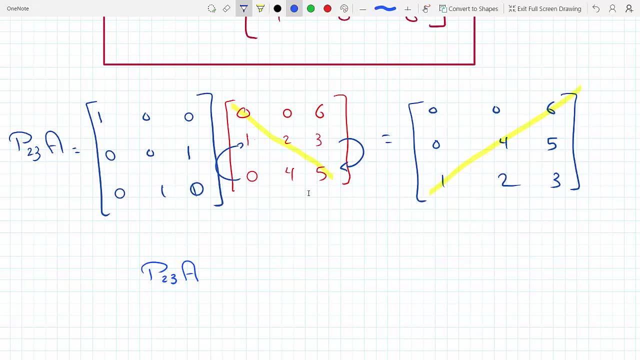 So I'm trying to switch the columns of A And what I'm going to multiply it with. I'm going to multiply it by P13. Because if I multiply on the right that would switch. I would want the third column to come first. 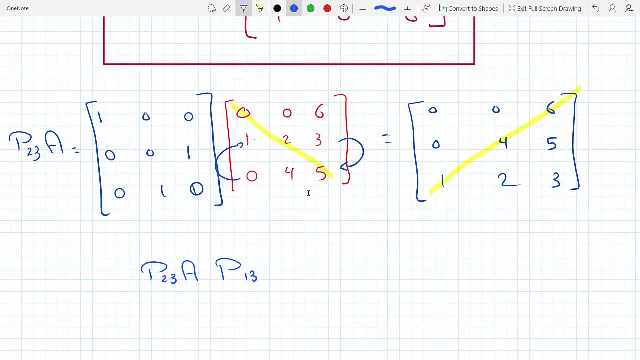 And the first column to come first And the first column to go last. Right, Yeah, So then I would take my end result, which is So: P23A is the above matrix in blue: 006 times 0, 4, 5, 1, 2, 3.. 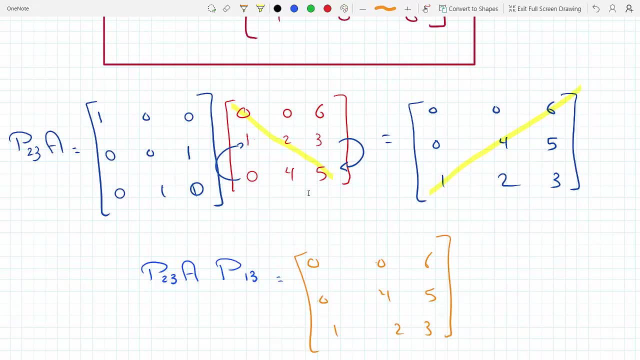 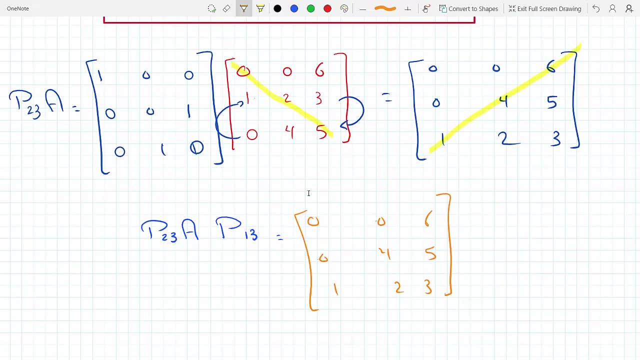 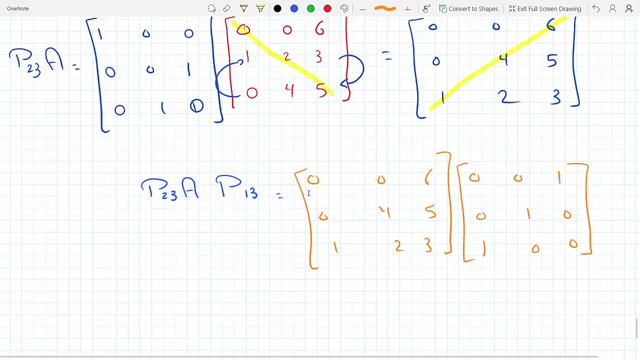 And if I multiply that by P13.. So that's exchanging the first and the third row of the identity matrix, So 001, 010, and 100.. And if I do that, what will happen is I will get.